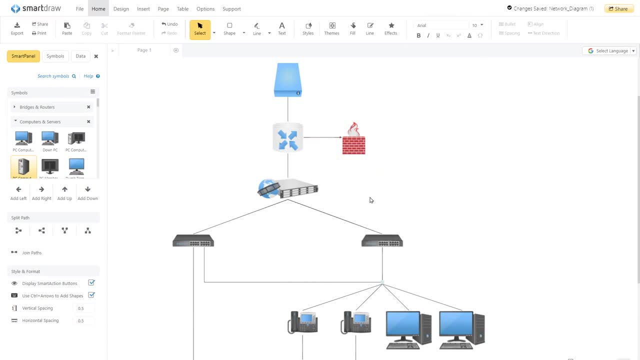 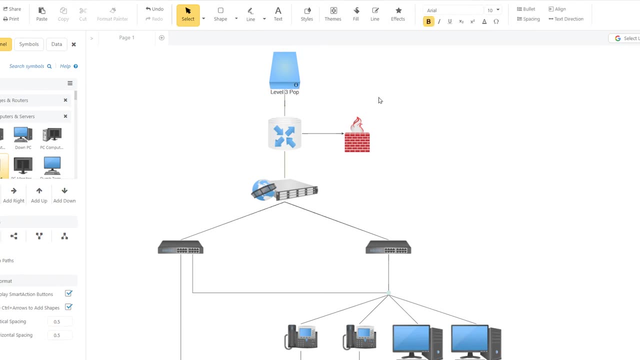 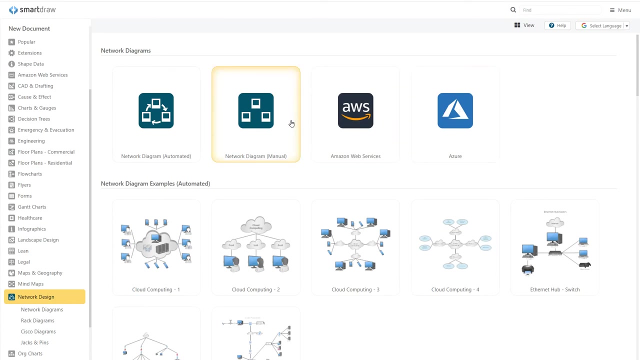 an arrowhead to indicate direction. Now we want to add labels to our symbols. With a symbol selected, simply type to add a label, Or double-click on a line and type to add labels and descriptors to these connections. If you need flexible line drawing, you can choose the manual network. 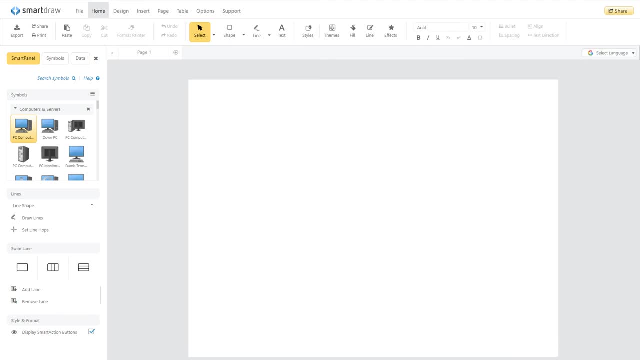 template and you'll be able to add lines and shapes. that way, You can add a symbol to your drawing by selecting it in the Library and then clicking anywhere on the page. You can add more shapes using the traditional drag and drop method Or, once you've already added a symbol, you can add mixed size andστε exposure. 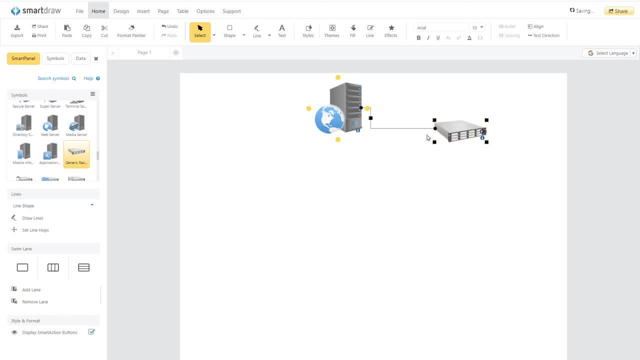 If you want Li mode to be in the line art form, you can select part shadows up, then choose Karadet to be in the hollow surface lens or add a image to the complicates added a symbol. you can add new ones by drawing a line and choosing a symbol from the auto. 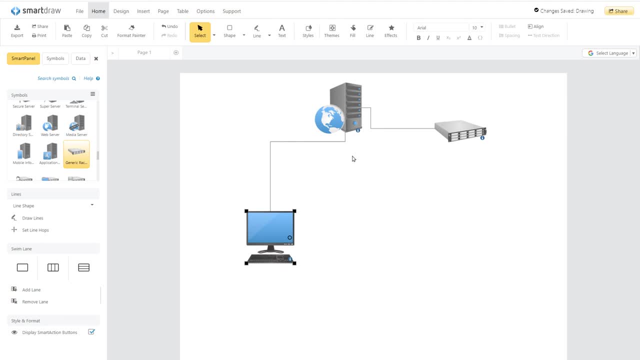 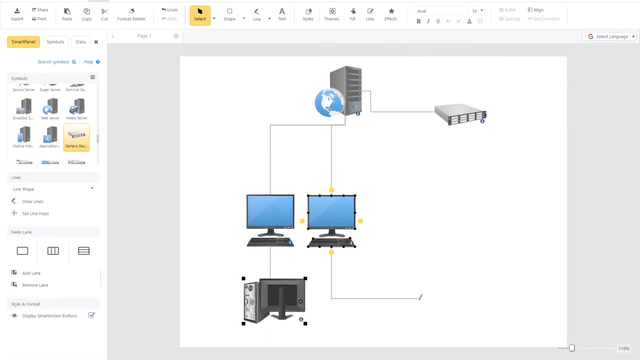 prompt that appears. This menu is pre-populated with the most common symbols for the selected diagram type. The options will change over time to symbols you commonly use, so you'll always have what you need at your fingertips. Add shapes in any direction and easily connect. 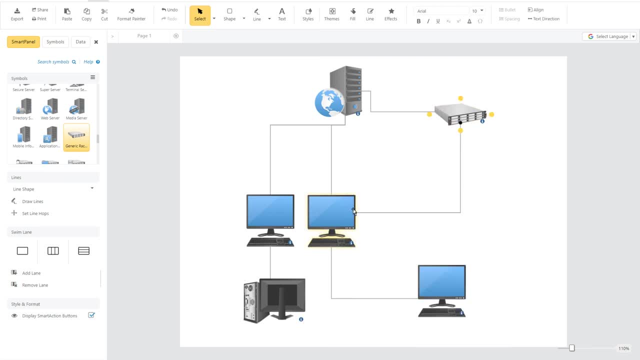 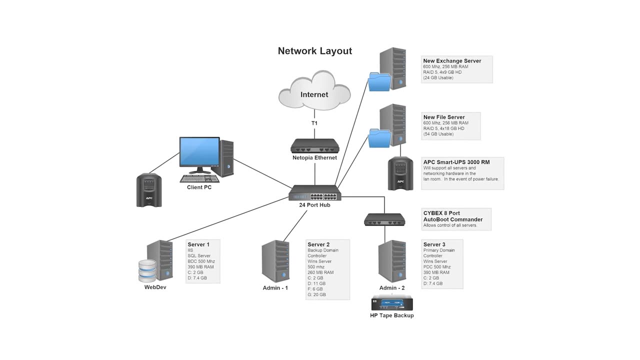 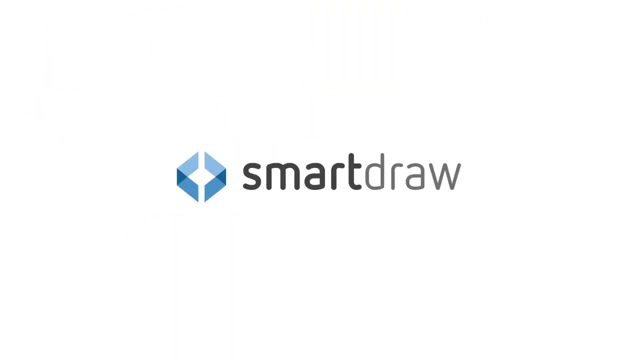 existing shapes to each other using the Same Line tool. You'll have more control over how long your lines are and where you add shapes. A network diagram is an ideal way to share the layout of a network visually, And nobody does it easier or with better results than SmartDraw. 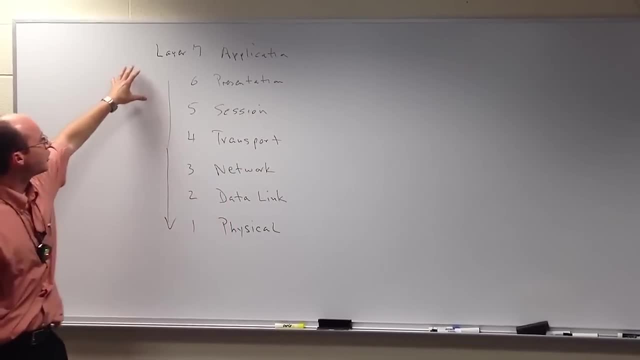 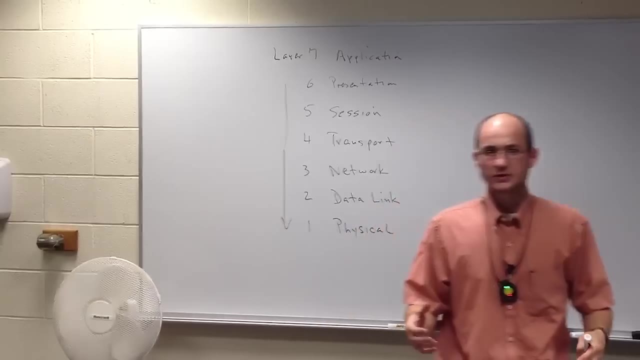 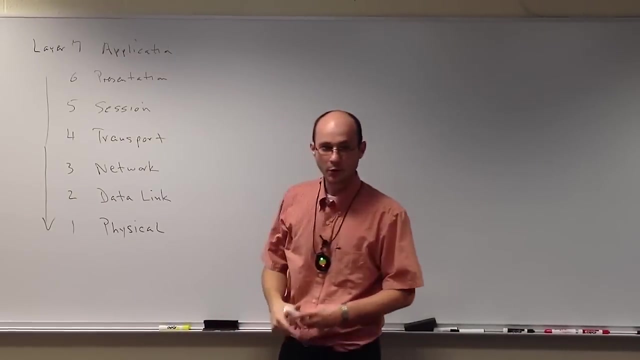 So, like I was telling you guys, the OSI model is more of a reference, a guideline to help us delegate responsibilities, to help us understand what the communication process entails. And so I had you guys just list them out from top to bottom, but remember, the communication process entails: 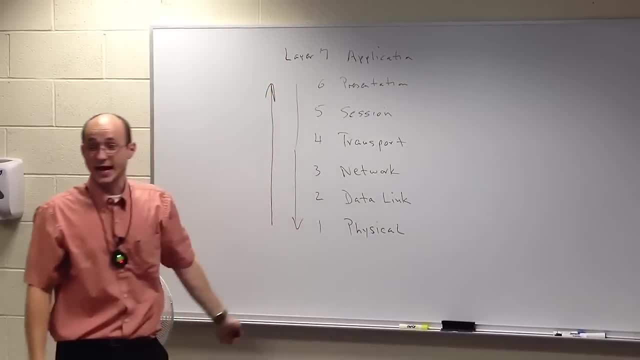 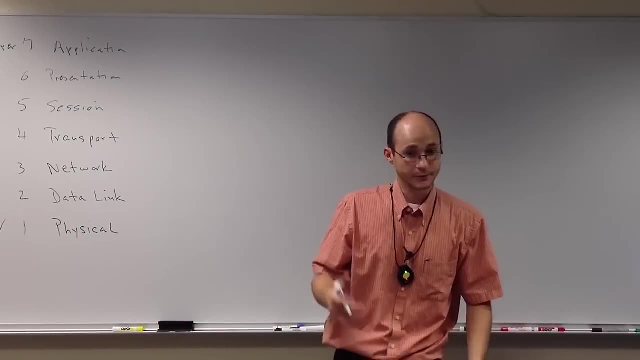 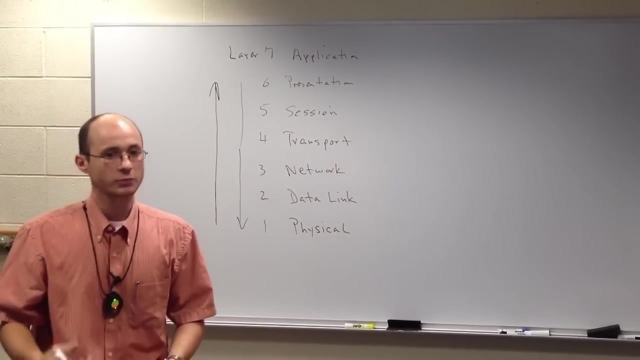 both directions: Going down the stack is what we call encapsulating, and going up the stack we call decapsulation. And today I hope to explain why the encapsulation process is very critical to the communication that is, to get the message from the sender to the receiver.